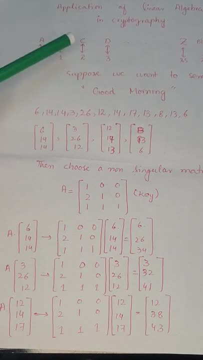 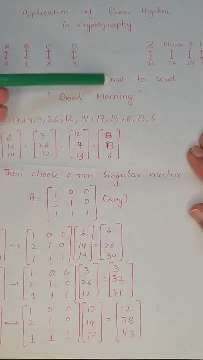 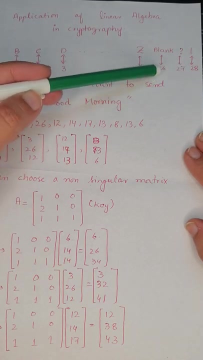 the value 1 and so on. you can see the alphabets are assigned different values. Similarly, if your text contains certain blanks or a question mark or exclamation sign, then you can assign similar in the same way in the different integer values to them. so for the time being we are sending a. 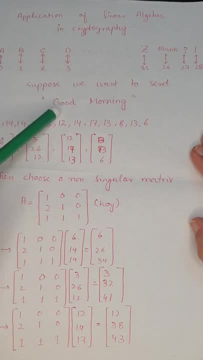 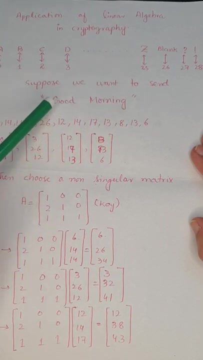 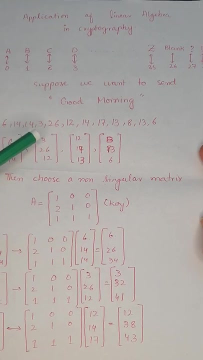 message that is actually composed of how many letters G double O, D, and then there is a blank. you can see then M O R N I N G. so the total total number of the alphabets including the space are equal to 12. all right, so i have written a g. 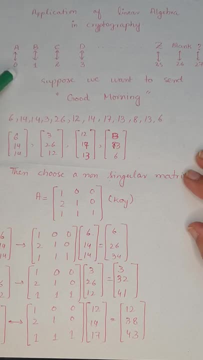 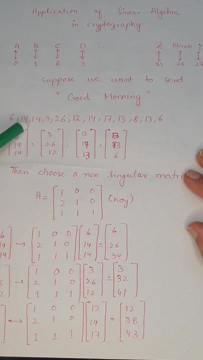 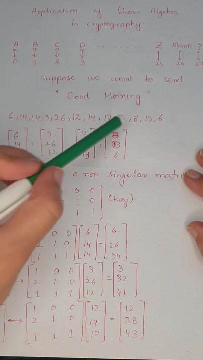 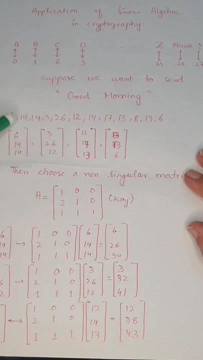 or assign the value. g is equal to 6, as per the order selected in the above, so g equals to 6 and similarly, all is assigned 14, then again 14 and d is assigned the value equal to 3, and so on. you can see. i got this sequence of the numbers from this arrangement that we have chosen. 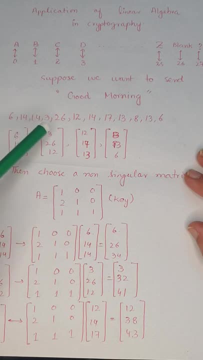 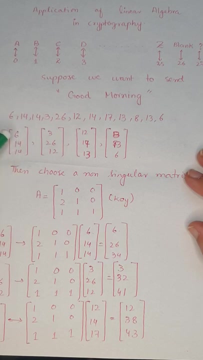 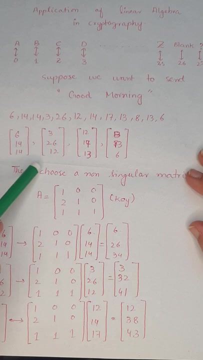 after doing that, we have broken our this list into the column vectors of a3 elements. so, all right, we have actually selected our column vectors. having three entries, we can choose the column vectors of the larger entries, but just for keep our her calculation simpler, we have chosen this sequel. 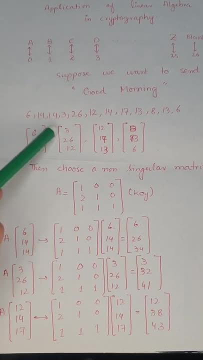 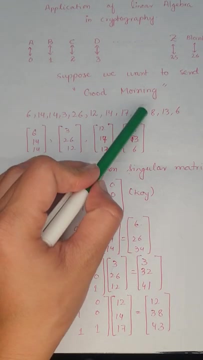 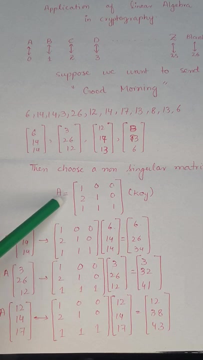 the next task is to encrypt these messages. so basically this is my message one. this is my message to message three and message four. basically i have actually broken down my original message into the smaller vectors. then i am going to choose a key. let's say it's matrix or the- preferably square- matrix and the proper vector we are going to use to encrypt. it is equal to feet, to the smaller vectors and so on. sorry, this day you want to do most of it, but i do not bother checking the message. i will understand how much i have added, which is normal because lots of individual data has not been classified into the column Stadium here, so i will do that. just in practice, however, everything looks exactly the same, so let me finish this problem byえver do it now. i will just input this new column here. this is an overwhelmingly check for the number of elements, the those that are. 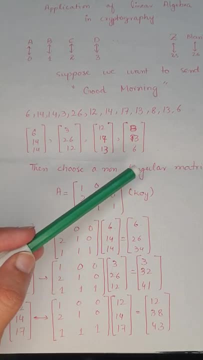 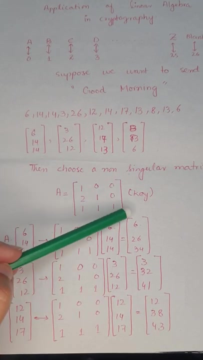 of the square matrix should be like that. it should be the singular matrix. why? because if I am choosing a phenomena of the multiplication for encrypting our message, then for the decryption, or while decrypting my message, I have to find the inverse of the matrix. so that's why the single, non singular matrix is chosen. you. 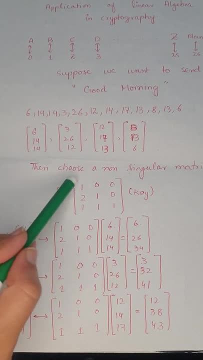 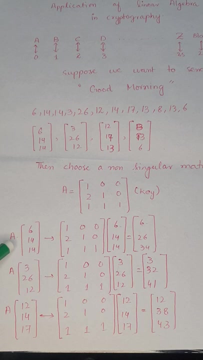 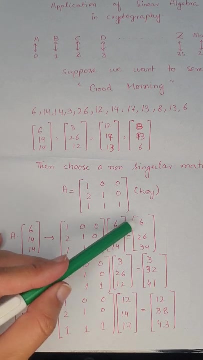 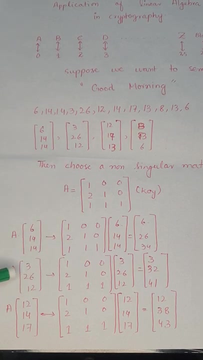 can also see later on how it will work. so I have chosen a very simpler key for encrypting my message and then I have written, or I have done what the matrix is actually being multiplied with my first message and it results into 6, 26 and 34, all right. similarly, the next message is again multiplied with the key. 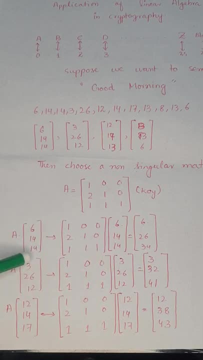 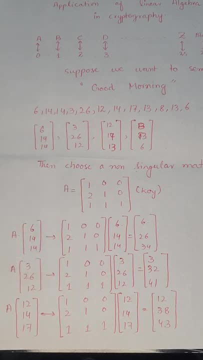 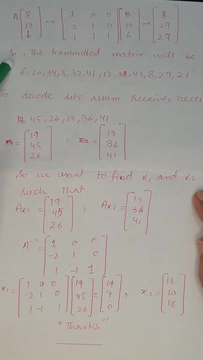 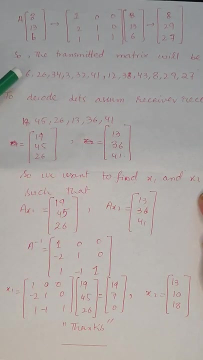 I will multiply all my four messages with the key that I have chosen for the encryption. now you can see over here: the messages that are now ready for the transmission have been transformed into some other messages and this sequence. if you try to decode this, decode this sequence, then you can see 6 was. 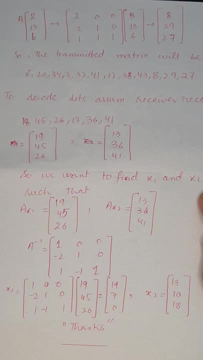 corresponding to G though. so the first letter that will be that you can predict is G. that is all right, but what comes next? it's 26 and 26. as we can see from the previous encoding scheme, 26 corresponds to blank, so it will cause as, or it can be written as G, then blank. so 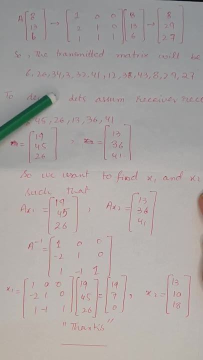 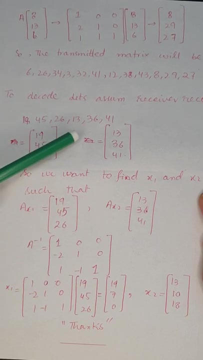 this is actually not the original message. all right, it has been hiding and it has been encrypted. now we will see how the receiver can decrypt this message. one of the cryptography rule is that the key that is used for encrypting the message must be known both to the senders and the receivers. so the 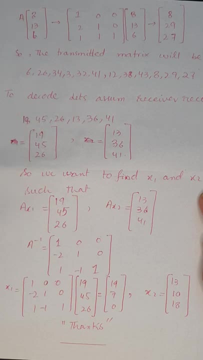 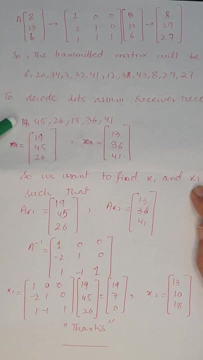 receiver, after receiving the message, can decrypt it easily or decode it easily. all right, let's assume, rather doing this sequence, let's say, the receiver actually receives this sequence. I have chosen this sequence so that I can do it in the smaller steps, but you can also take the same approach for decoding this message.